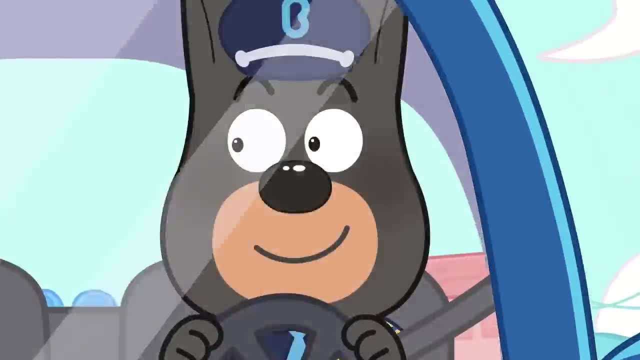 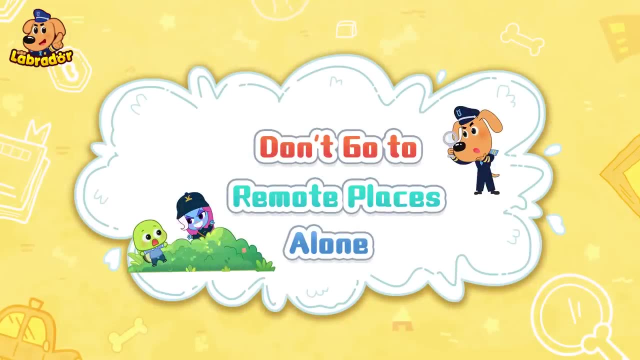 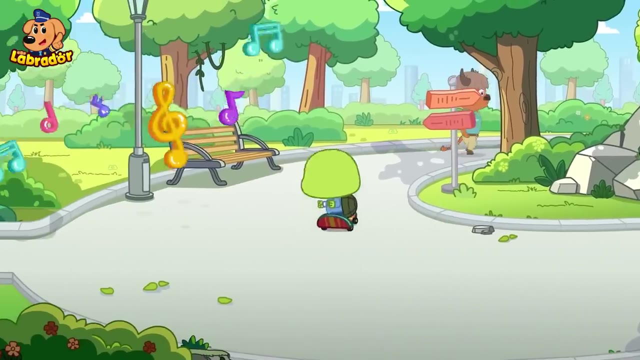 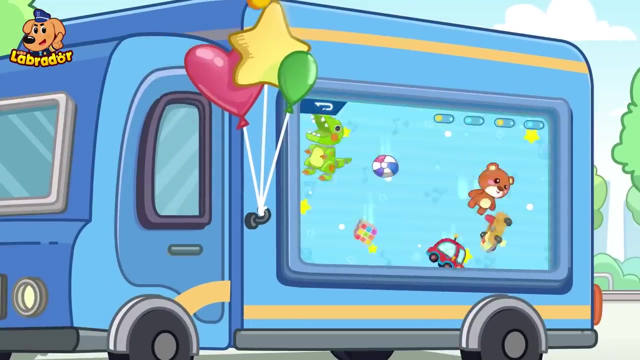 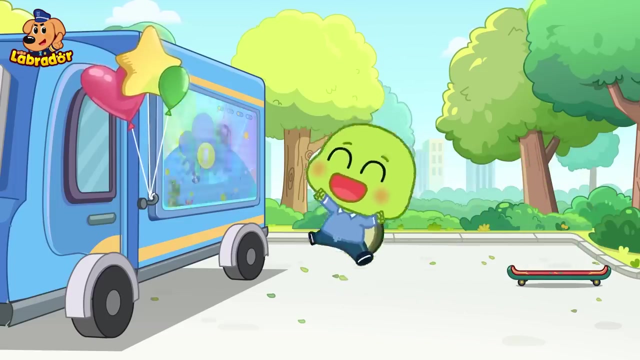 Go, go, go go. Let's go share it. Labrador, Don't go to remote places alone. Yahoo, Play games and win a prize. Amazing toys are waiting for you. Wow, They're all my favorites. I'll do it. 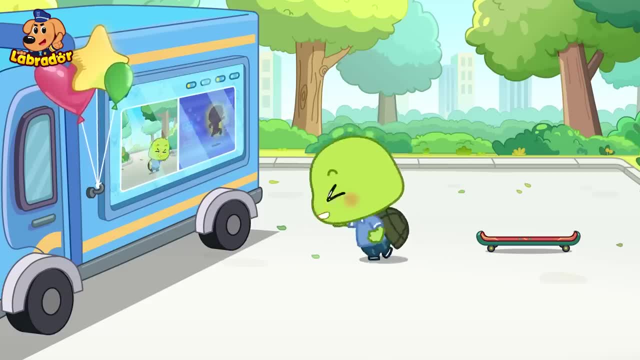 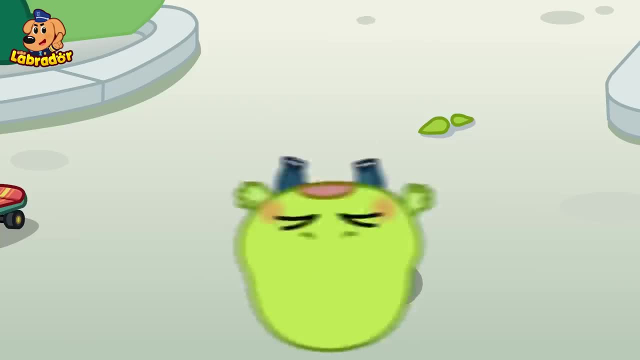 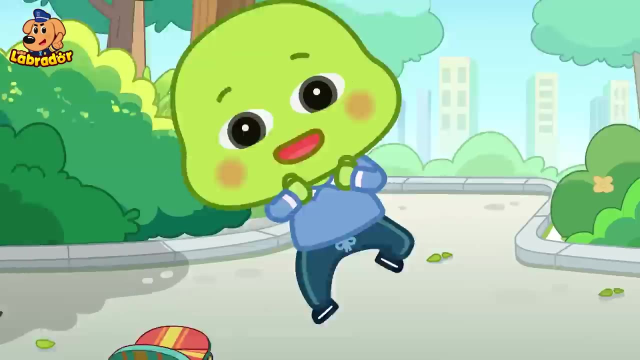 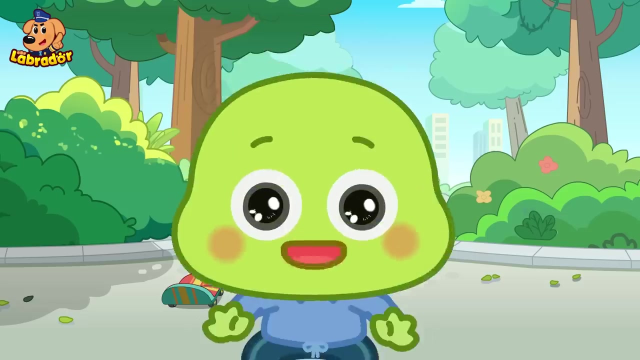 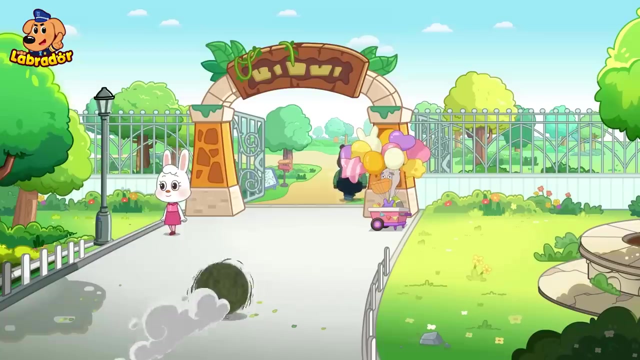 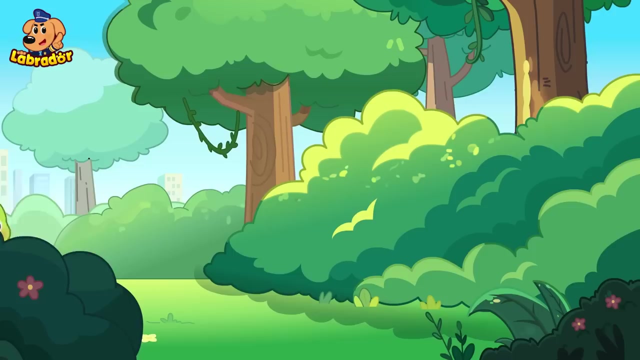 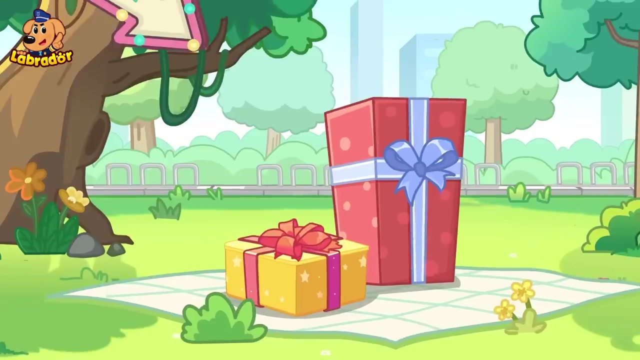 It's starting Spin Perfect. I can't believe it. Congratulations: You won a prize. Wow, It's so cool. Please follow the arrows to collect it. Let's go This way. Where am I? Wow, It's my prize. 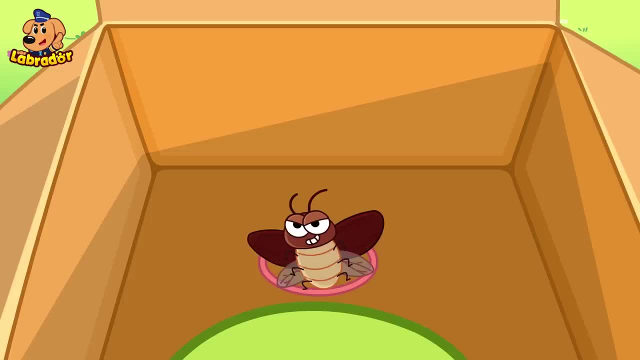 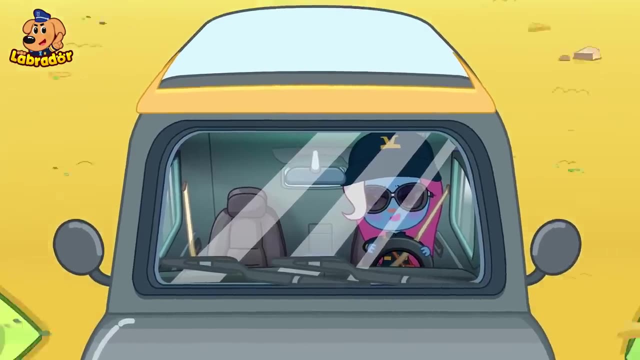 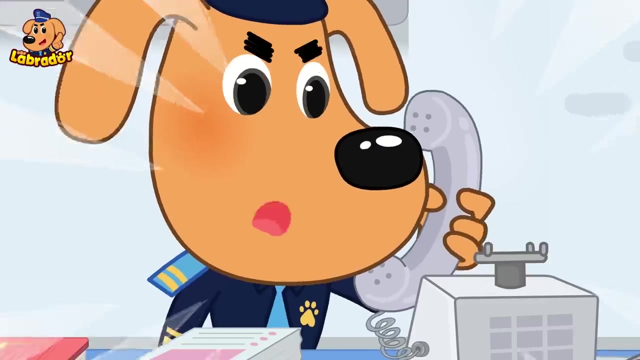 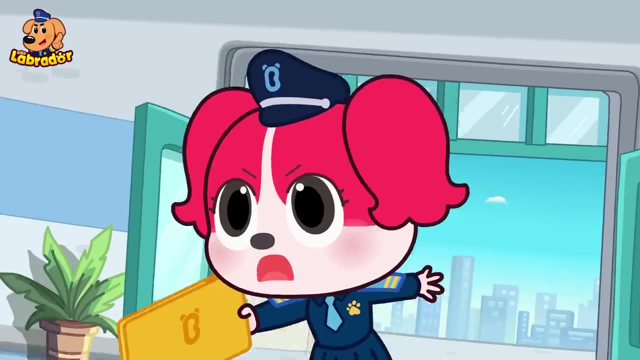 Help, Help, Help, Help, Help Help. Oh, the kid fell for it. Let me out What Another child is missing. There's a third one. It's horrible, sont 7!. All the missing children play a dance game. 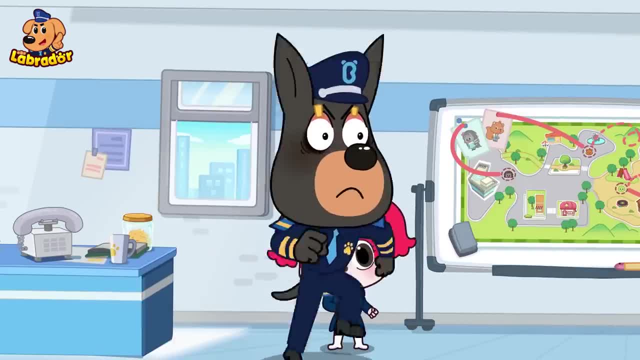 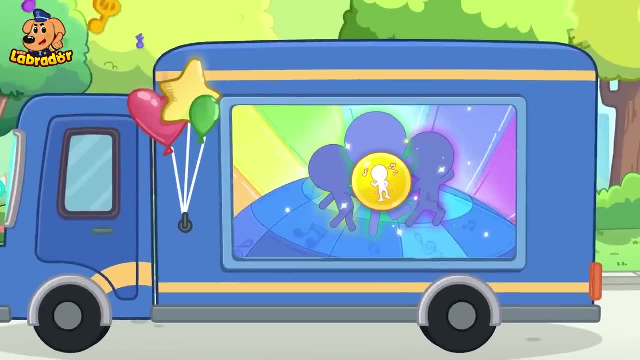 There must be something up with this game. You have something to do inside. Let's go Saudi Arabia. We have to leave Friday. New York: Oh Hi, Play games and win a prize. Amazing toys are waiting for you. I'll do it Start. 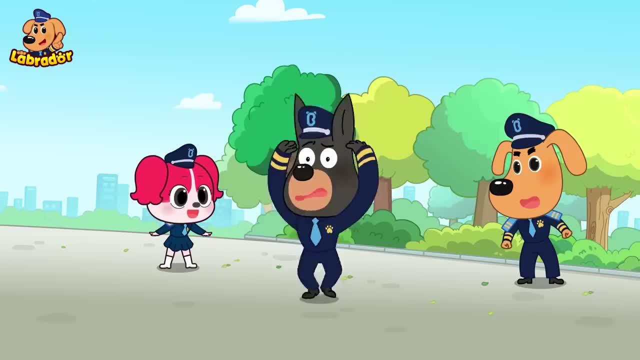 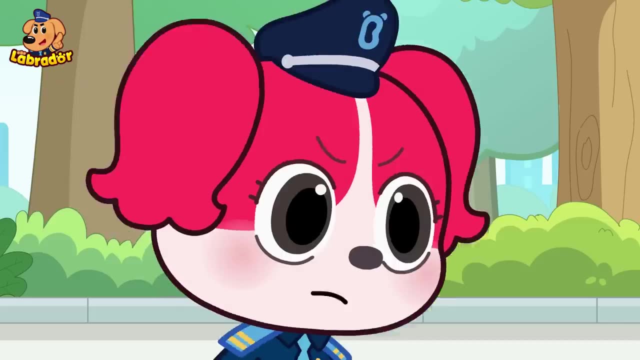 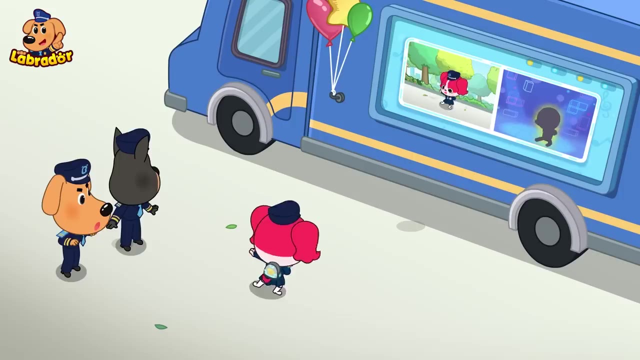 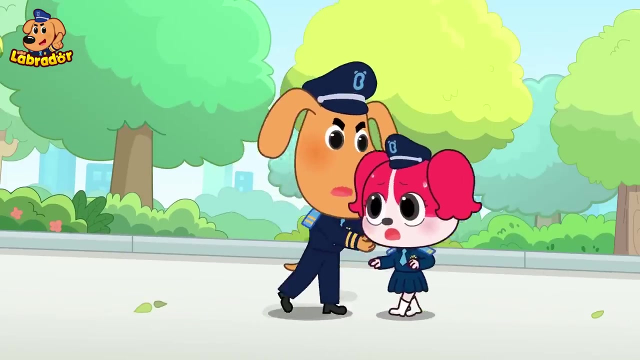 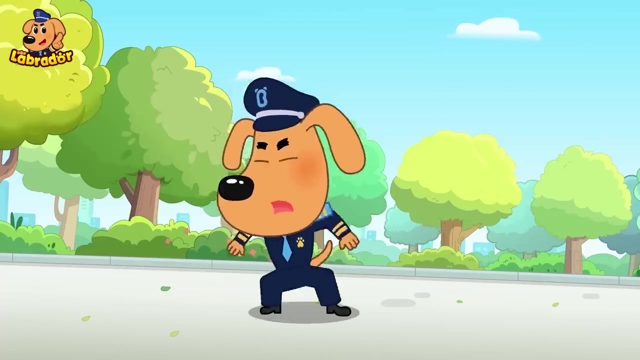 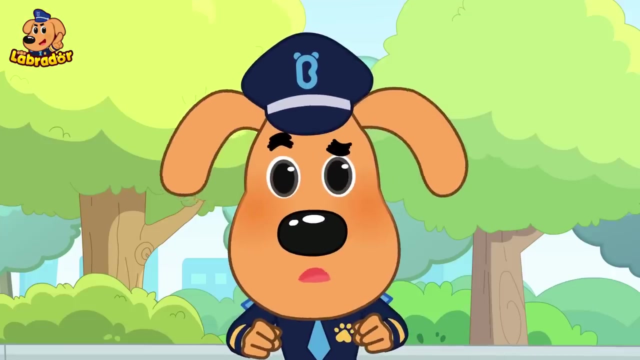 Oh no, I can't keep up. I'll try. Well, it's getting faster, I can't keep up. Careful, I'll do it from here. Perfect, Even with those moves. Congratulations, You have broken the record. 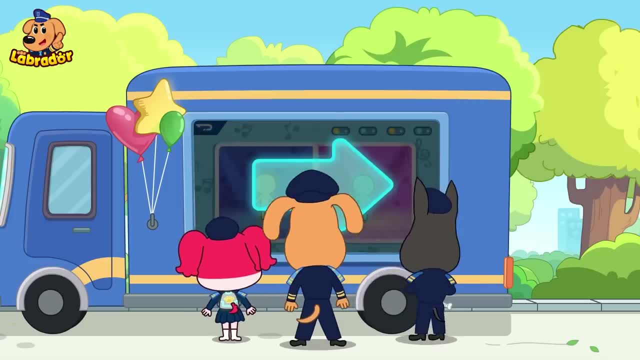 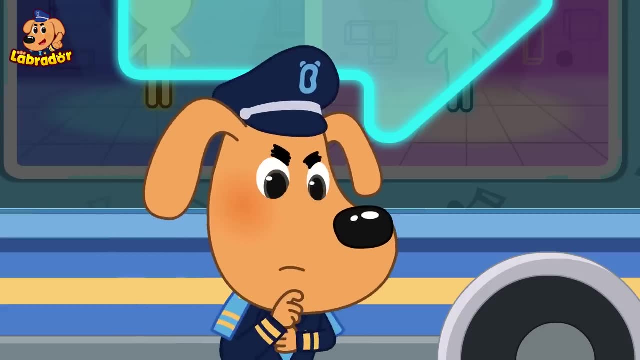 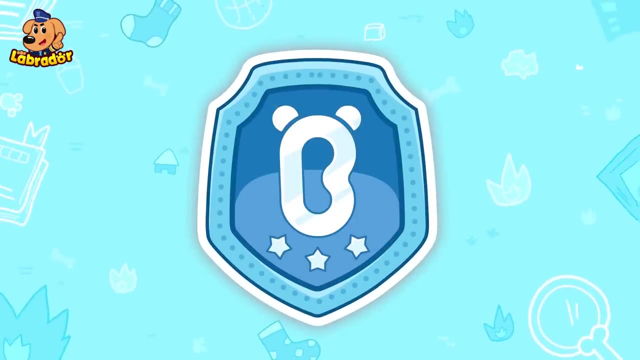 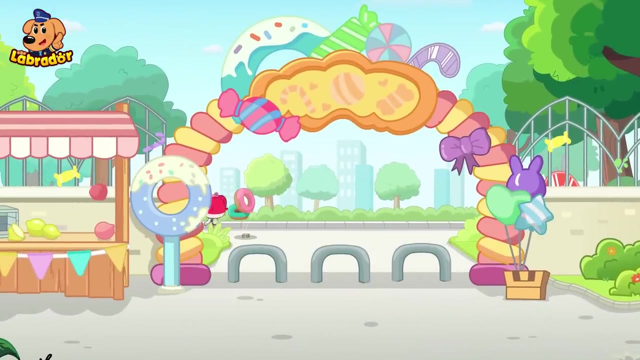 Please follow the arrows to collect your prize. Come on, Let's go. Woohoo, It's way too easy for a big prize. It must be a trap. I have an idea. It's here, Dobby, let's go. 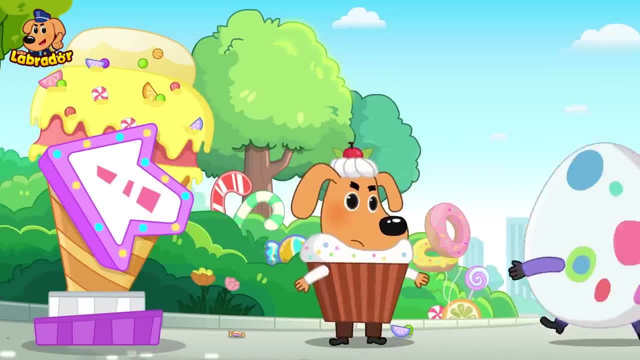 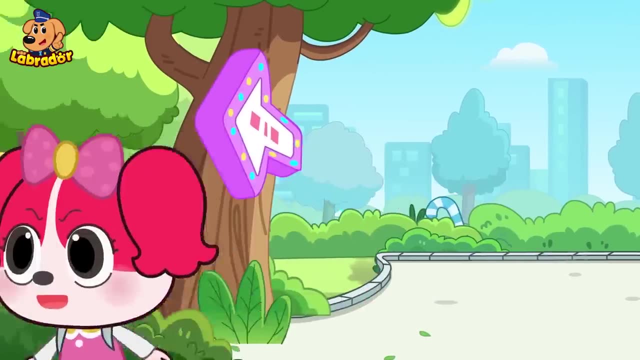 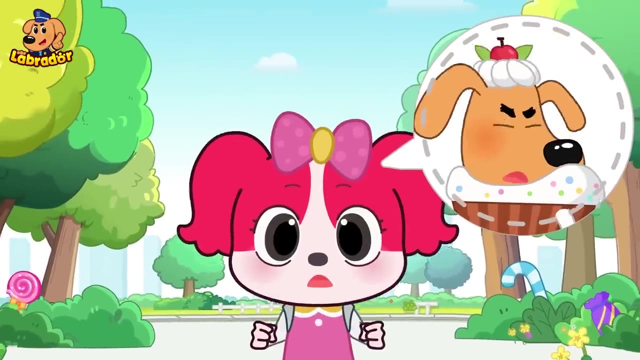 This way, Let's go Okay. Huh, Giving away prizes in such a remote place like this, Another fool's coming. There's no one here. Someone's luring children to remote places to collect prizes from winning a game They could be nearby. be careful. 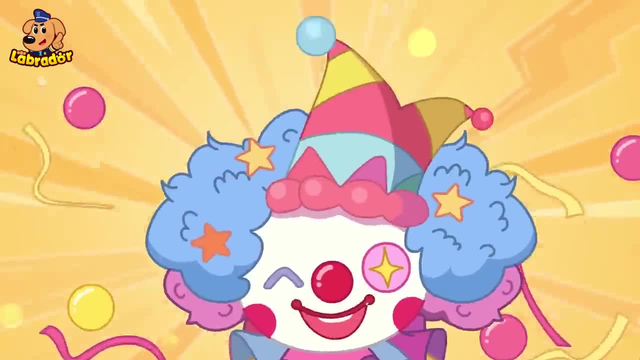 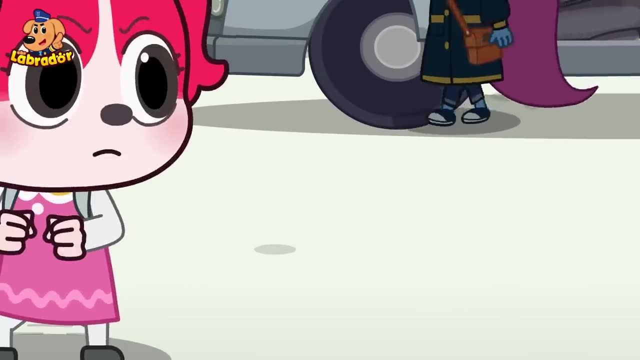 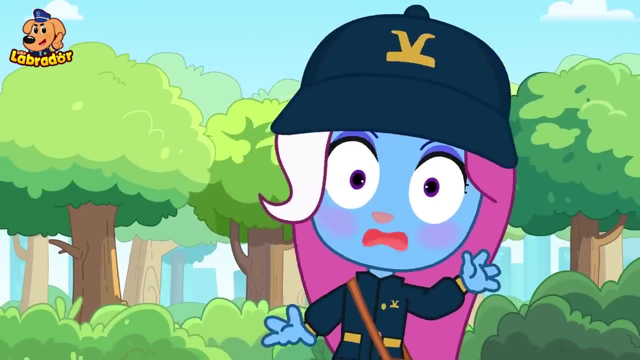 Wow, So many prizes. Huh Ahhhh, D시는, Help, Come with me. I've been waiting for you, The police, You're the one who tricked the children. You're under arrest. Now you got me. 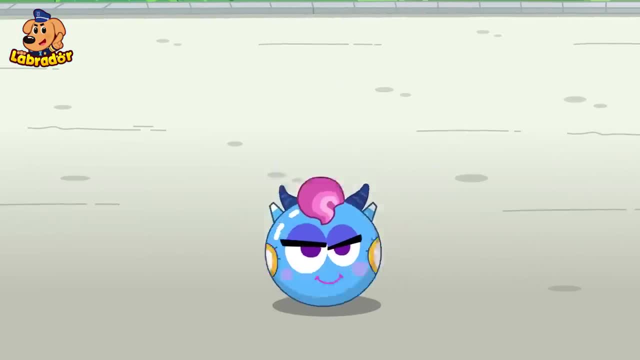 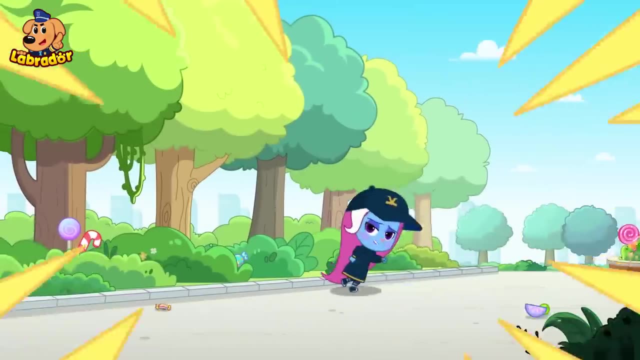 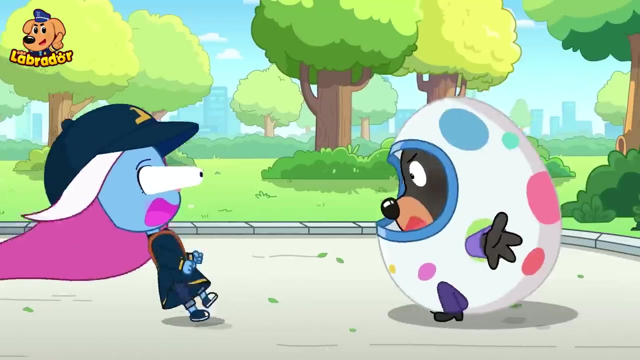 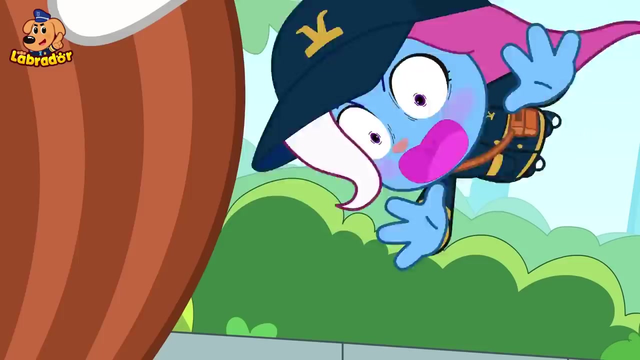 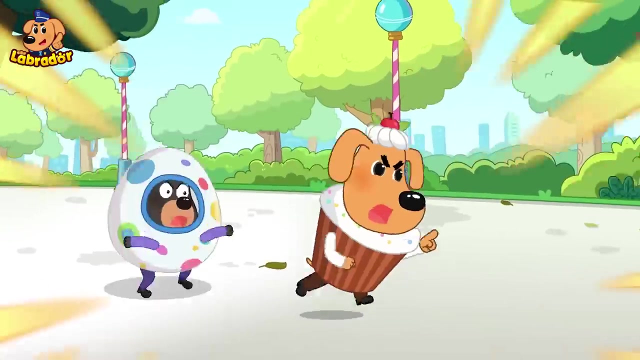 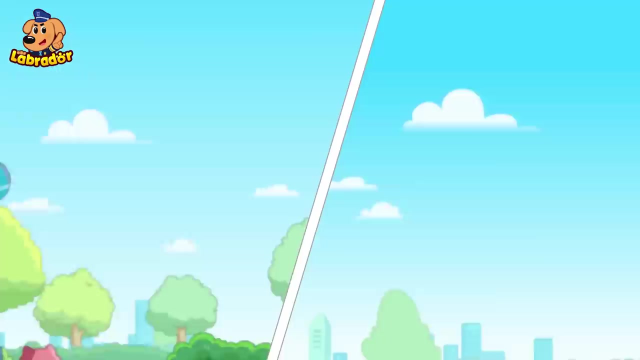 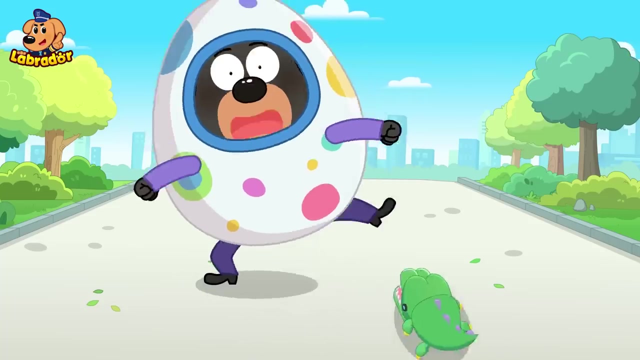 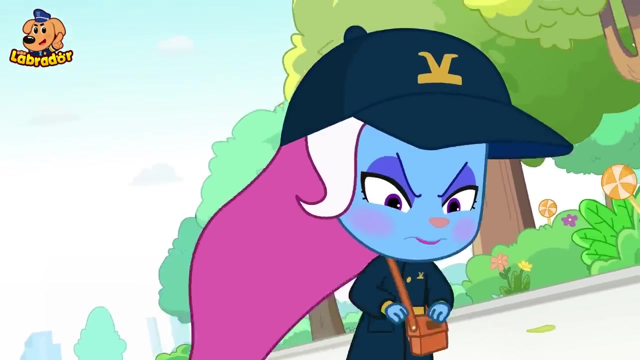 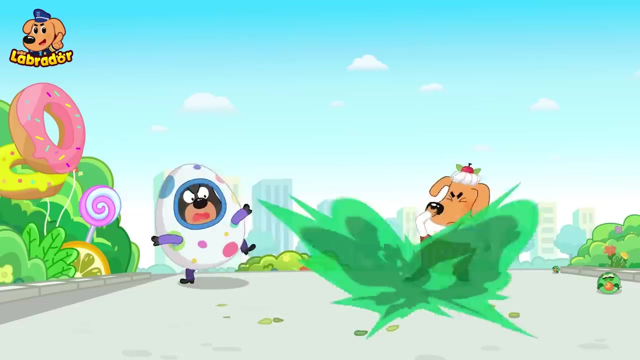 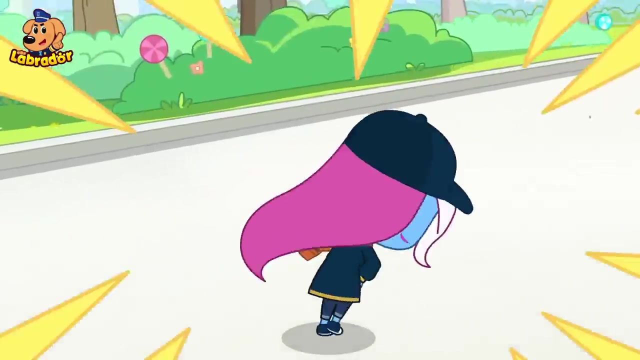 Hey, Where did she go? You'll never catch Dr Anto. Stop, You can't run away. See, Take this, It stinks. Looks like my stink bombs are quite useful. How about a few more? They are useful.